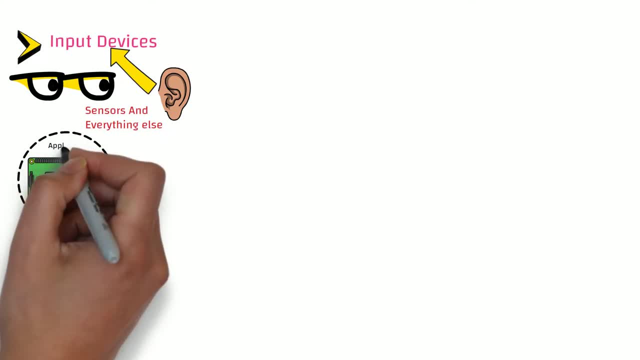 Since the hardware is custom built for the given application, so there is no use having sensors that we don't need. The following are some examples of the sensors used in embedded systems: Temperature sensor, Pressure sensor, Light sensor, Ultrasonic sensor, Humidity sensor, Accelerometer. 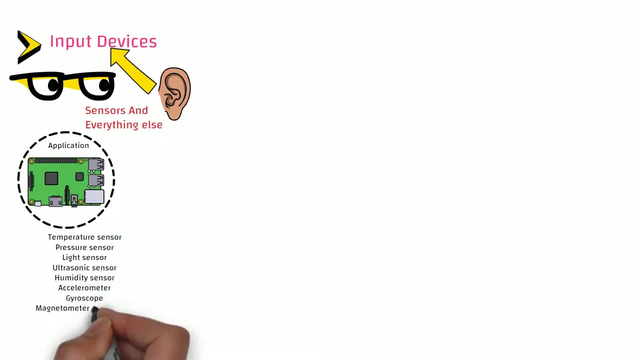 Gyroscope, Magnetometer or Compos. These are not only the inputs to the system, as inputs can also come from the user. For example, a button press event can also be an input, and data coming in through antennas or through wired means from external devices can also be considered as inputs. 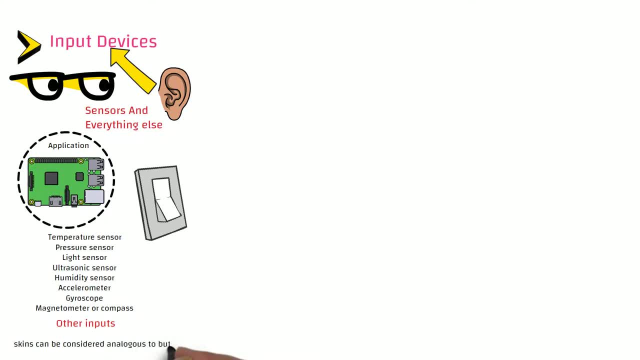 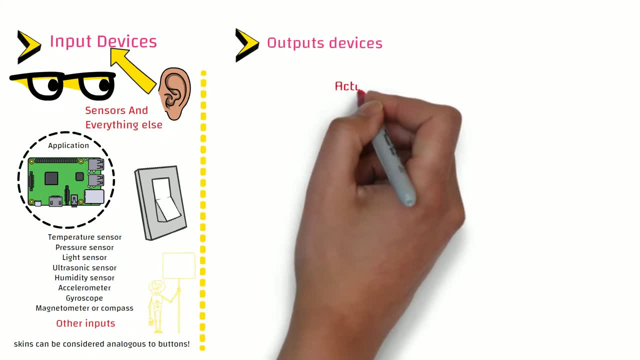 Coming back to our analogy of comparing humans to embedded systems, our skins can be analogous to buttons. Now let us look at some output devices. Actuators can be considered as arms and legs of embedded systems. They take instruction from the software and transform them into movement. 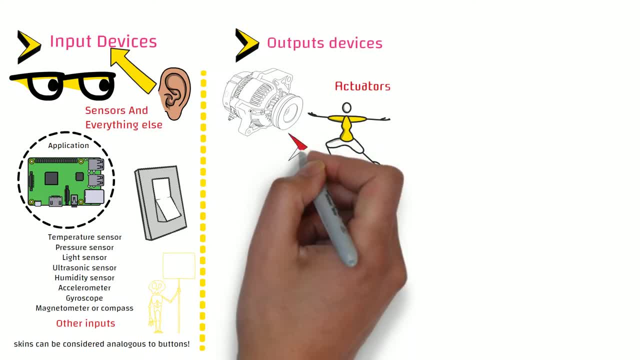 For example, a motor can rotate forward or backward depending on the instructions given to it via the software, which in turn will make the embedded system move forward or backward in the system environment. Actuators are largely found in industrial robotics and automotive applications. 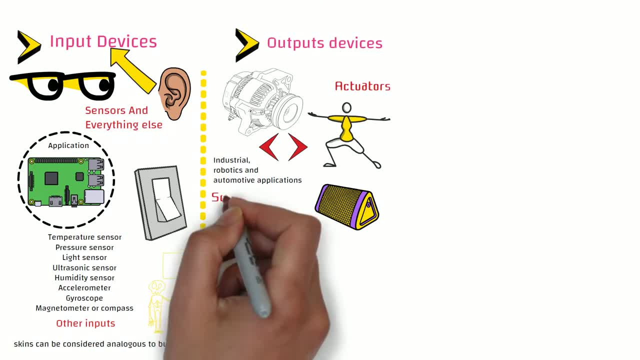 Another example of output devices can be speakers, through which you can play sound whenever needed, So I guess we can call them the voice of embedded systems. And, unlike humans, our embedded devices are also capable of producing lights, in the form of LCD screen and LED lights. 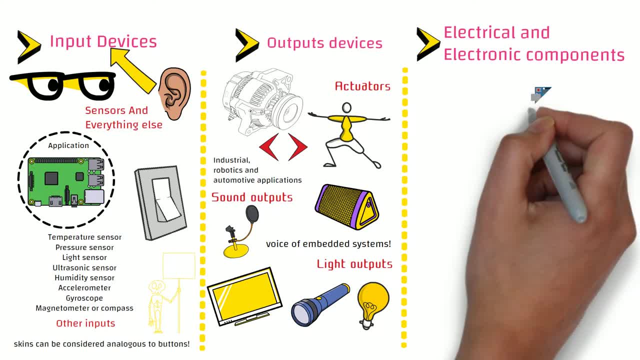 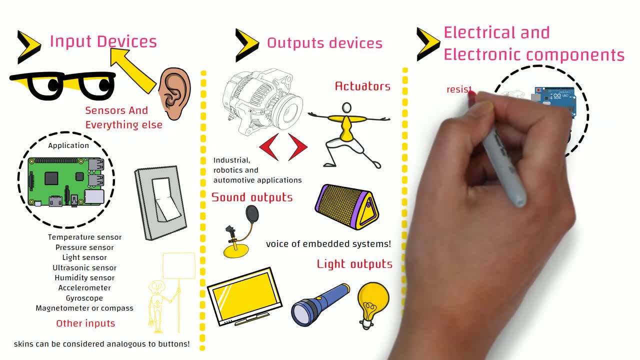 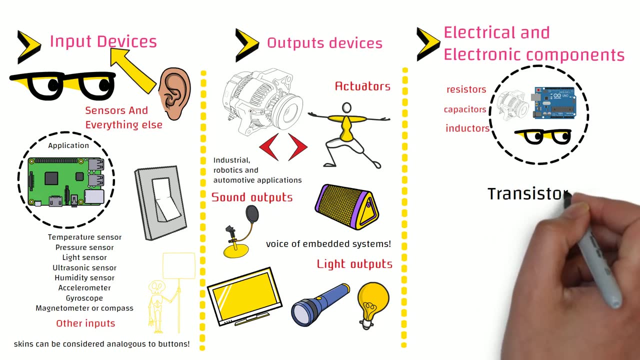 Next let's have a look at electric and electronic components. Connections between microcontrollers, sensors and actuators can require some passive components like resistors, capacitors and inductors. You will also see some active electronic components like transistors and diodes in a typical embedded system. 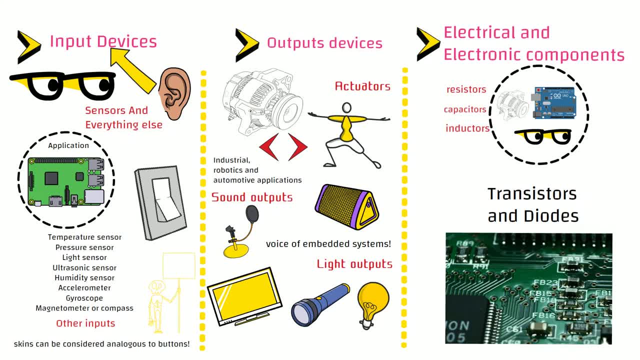 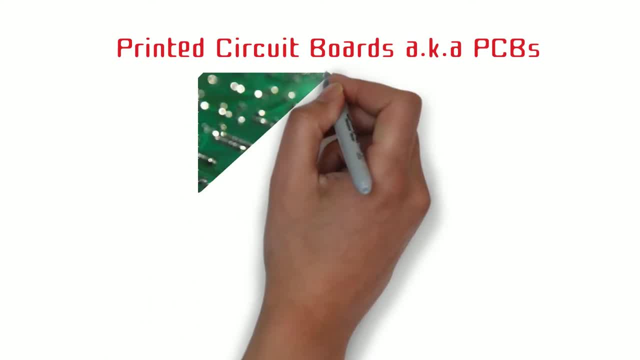 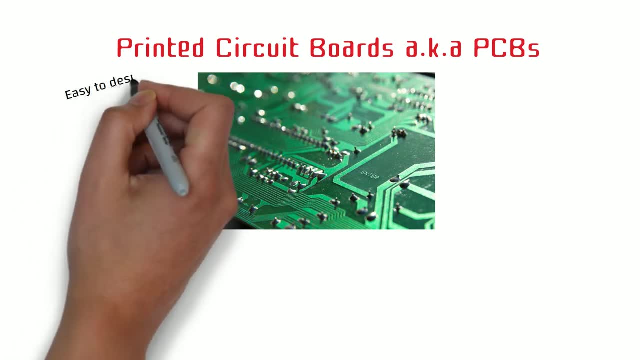 All these components will look alike from a distance, as shown in the picture. Printed circuit boards, aka PCBs, can be considered as the body which connects all the above-mentioned components together. Simple PCBs are usually very easy to design. You should be able to get started with just 10 to 20 hours of training. 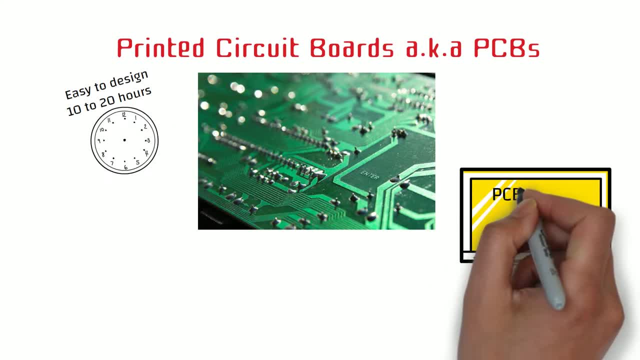 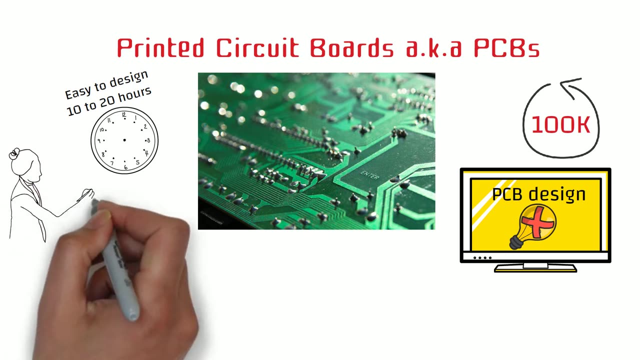 and then you can start producing your own personal PCBs. PCB design is beyond the score. However, we will probably make an introductory course on PCB design in the future once we reach 100K subscribers. Some say PCB design is an art. These are specialists that design high-performance. 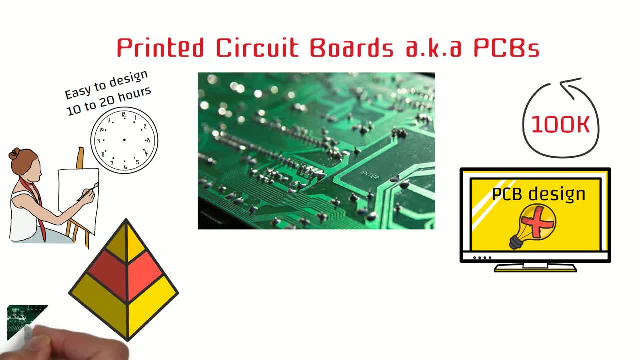 PCB boards with multiple layers to achieve smaller sizes of an entire board, at the same time keeping the product functionality intact. There are lots of external factors that can affect the performance of PCBs, like temperature, electromagnetic interference, etc. The job of a PCB designer. 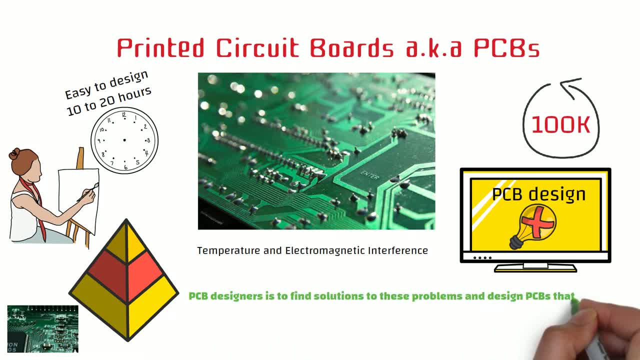 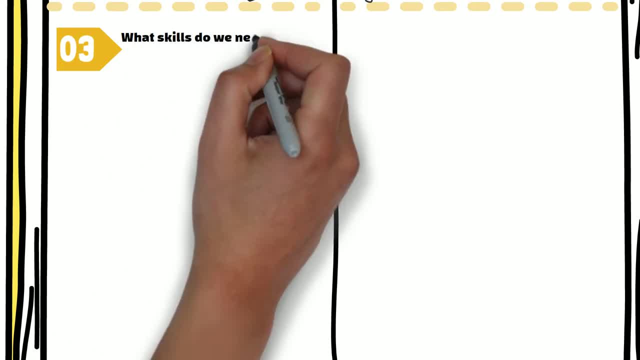 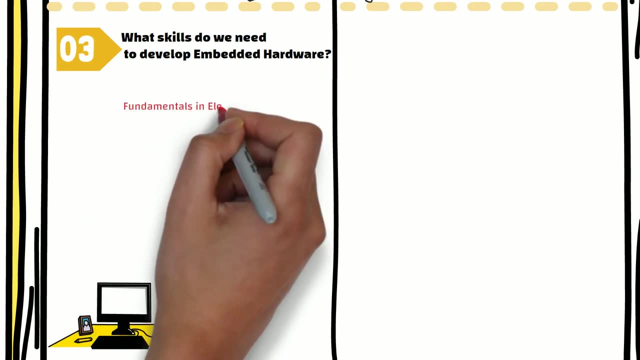 is to find solutions to these problems and design PCBs that give high performance. So what skills do we need to develop embedded hardware? An embedded hardware engineer must have good knowledge about fundamentals in electronics: reading datasheet and schematics. circuit design, design and analysis, microcontroller architecture, circuit debugging, PCB designing, electrical. 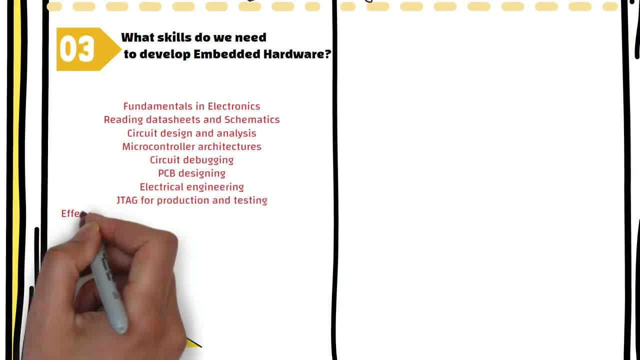 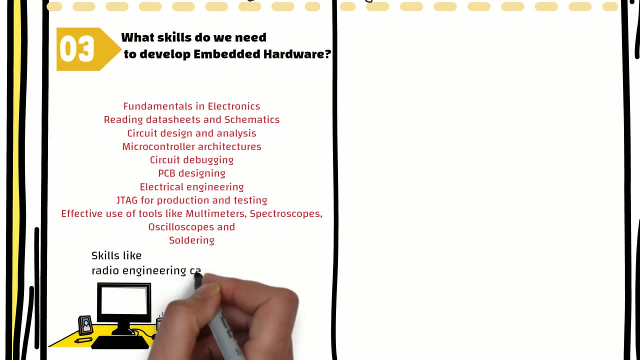 engineering, JTAG for production and testing, use of tools like multimeter spectroscopes, oscilloscopes and soldering. These are just the basics. Depending on the product being designed, other skills like radio engineering can also be needed For the beginners and hobbyists. 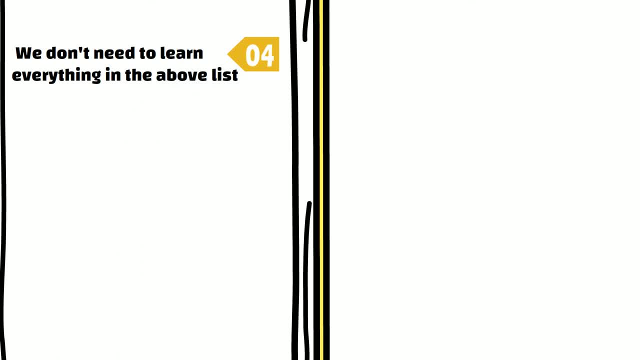 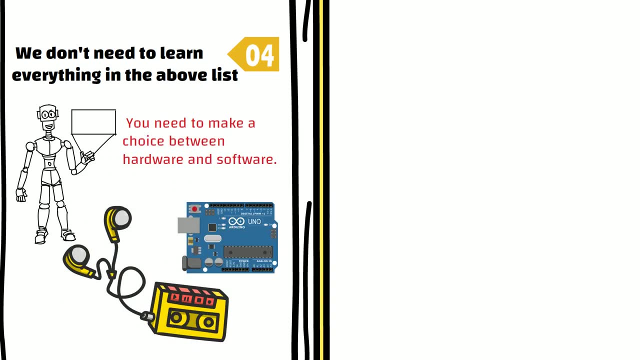 don't need to learn everything in the above list before we can start our journey. We can always use development boards to build our projects. If you wish to take up embedded engineering as your career, you need to make a choice between hardware and software, And then focus on one of.